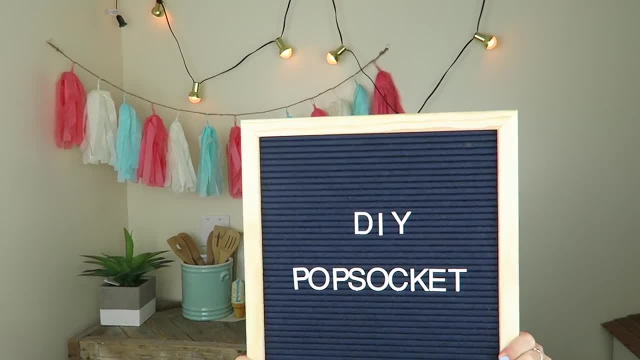 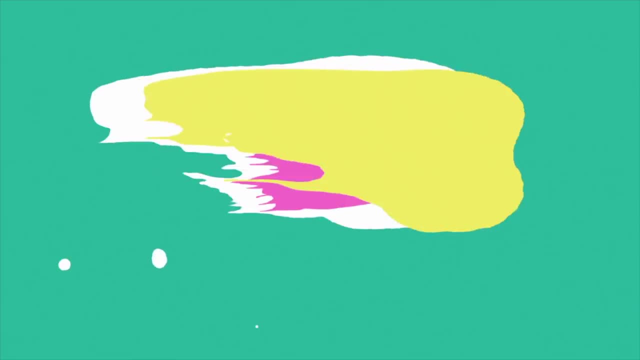 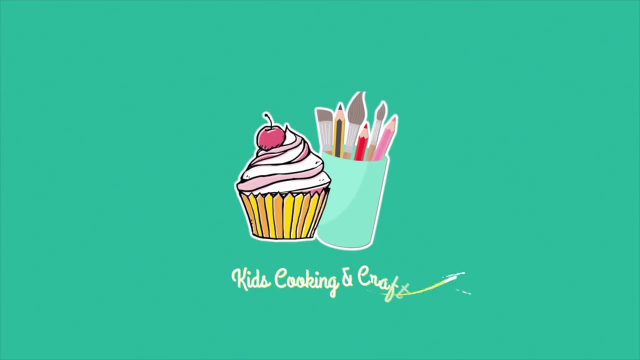 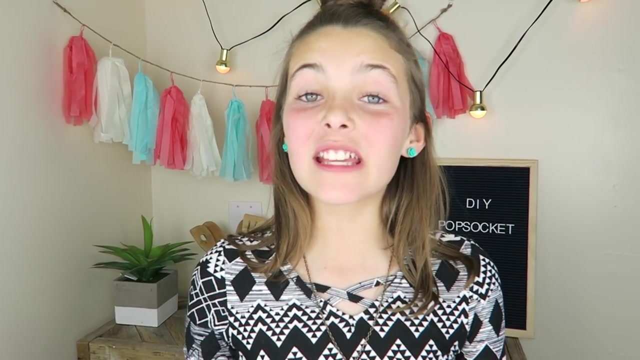 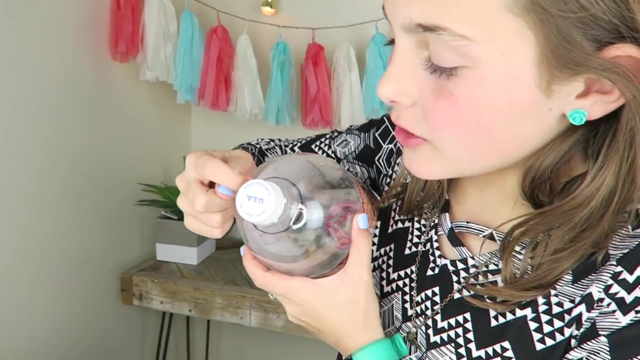 Today we are going to make a DIY pop socket- Pop socket. So a while back, we made a video about decorating pop sockets, but today we are actually going to make our pop sockets Using a bottle. As you can see, we have already drawn a circle where we are going to cut it. 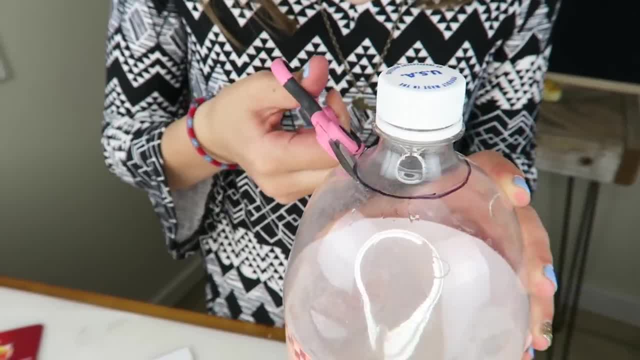 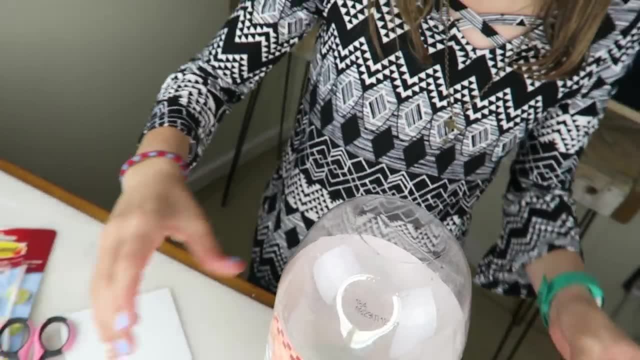 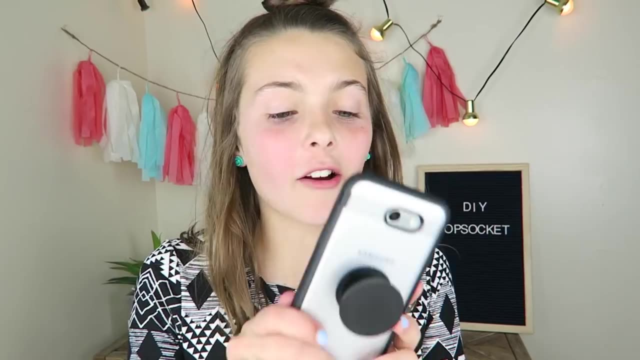 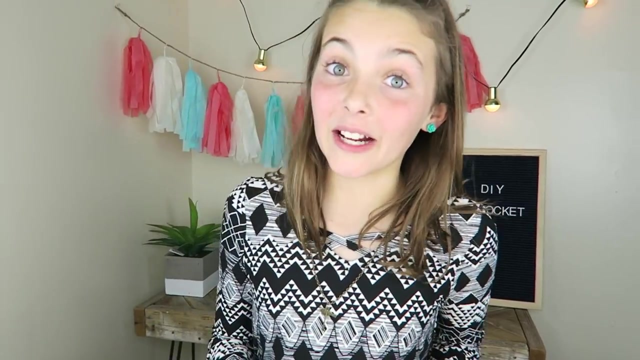 So let's do that right now. Check it out. It already kind of looks like a pop socket. Alright, check out my brother's phone. See his pop socket. This is kind of the same thing, Same shape as it. Alright, here we go. Now we have to put something right here to cover up this hole. 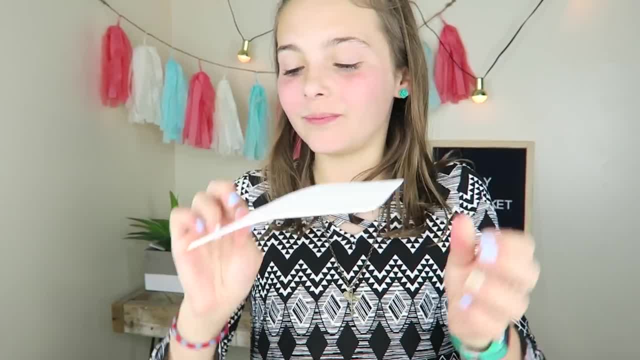 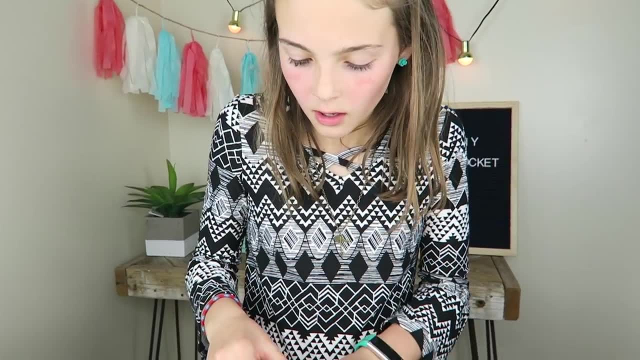 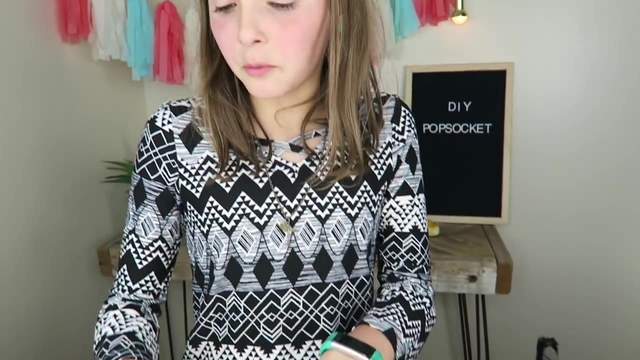 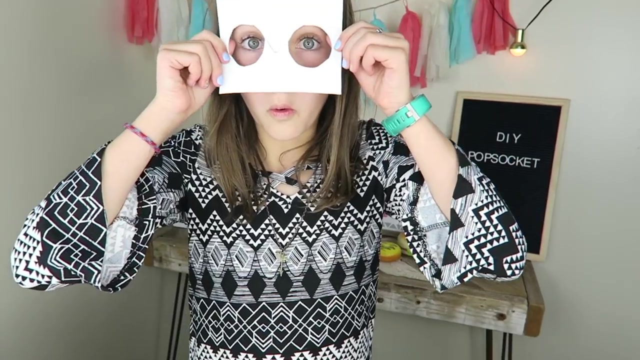 What we are going to do is use this white foam paper- I'm going to fold it in half to make it extra strong, And then get a cookie cutter and trace it with a pen, And then we just cut it out. Now we are going to glue these two circles together. 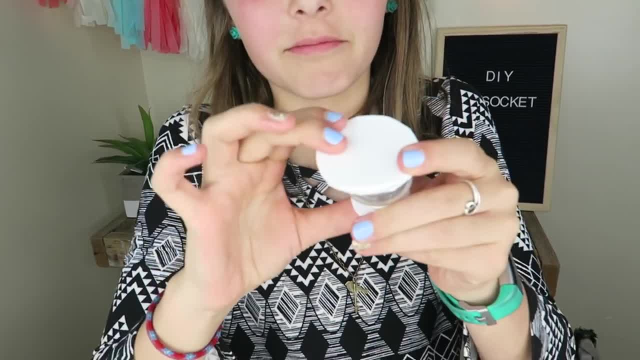 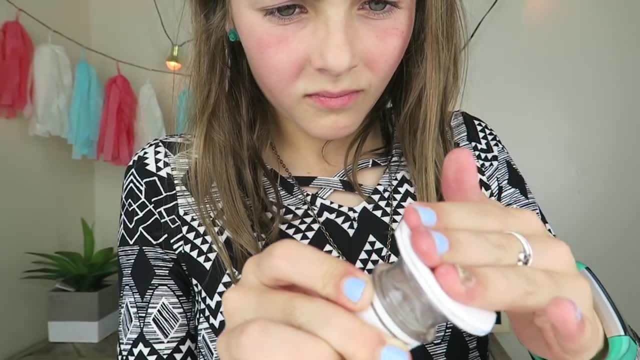 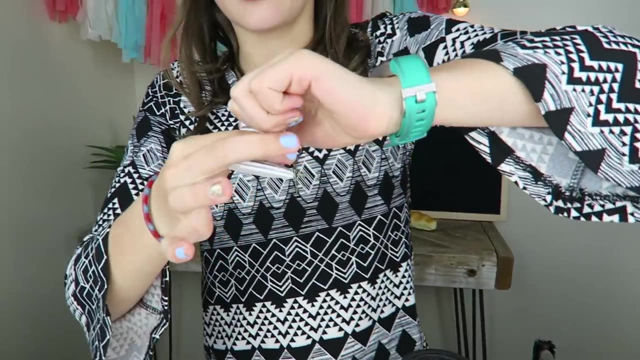 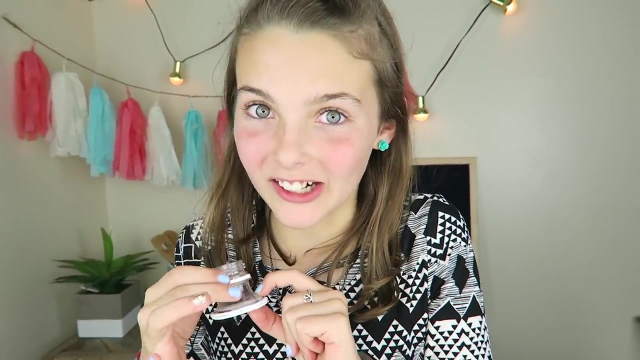 And now we are going to glue this one circle onto here, So it's just like that: Ta-da, Now it's sealed off. Here's the cool part. So we are going to unscrew this part right here And we are going to fill it up with glitter. 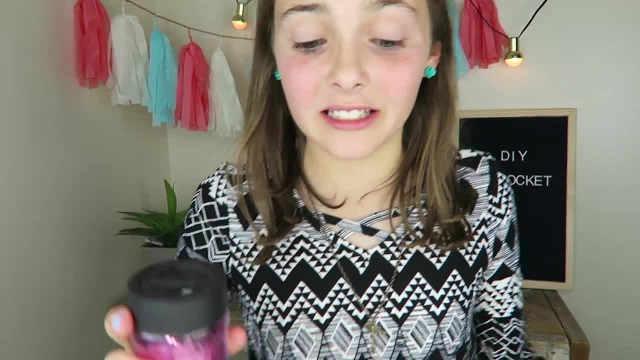 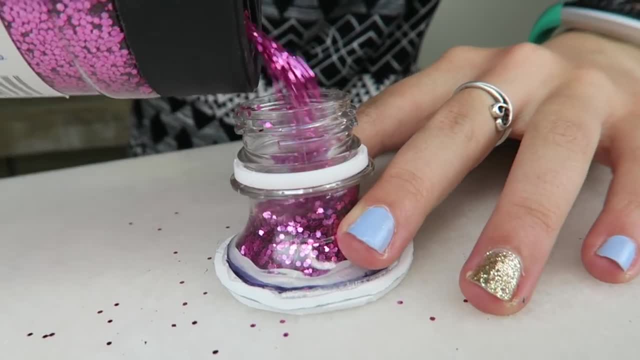 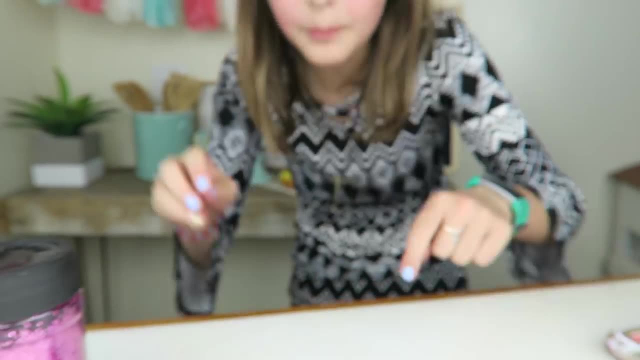 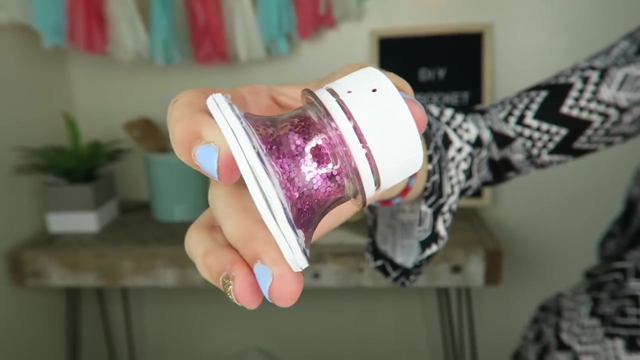 I'm using pink glitter, but you can use whatever color you want. As you can see, I didn't fill it like all the way to the top because I wanted it to like shift around, See, So I can like shake it. Now we are going to decorate it a little bit. 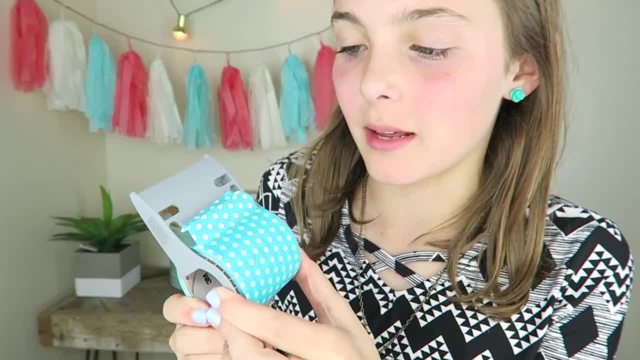 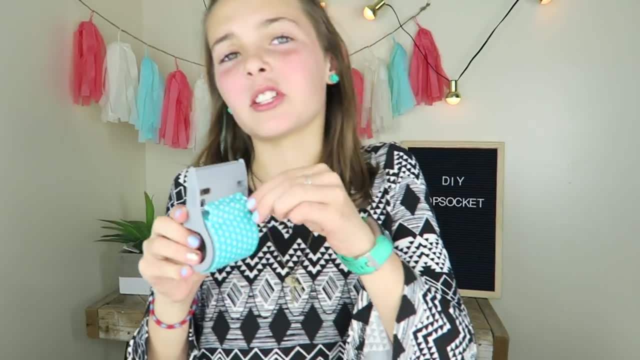 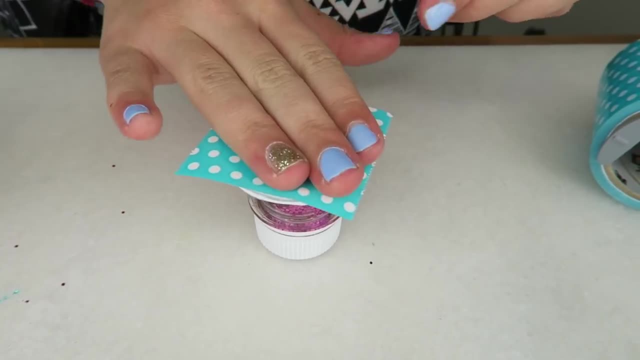 I'm using this white and blue polka dotted duct tape. You can use anything you want: Scrapbook paper, stickers, glitter, more glitter. But I'm just going to stick with this. Now, I'm just going to cut it to fit. 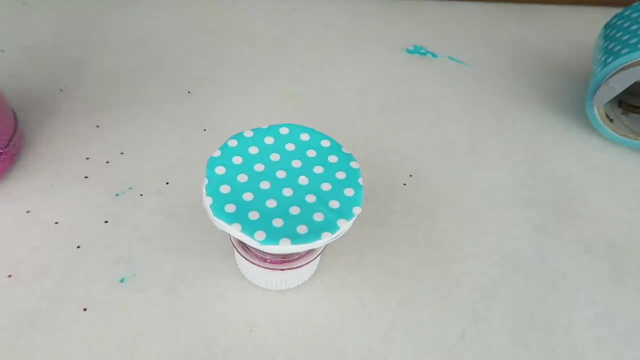 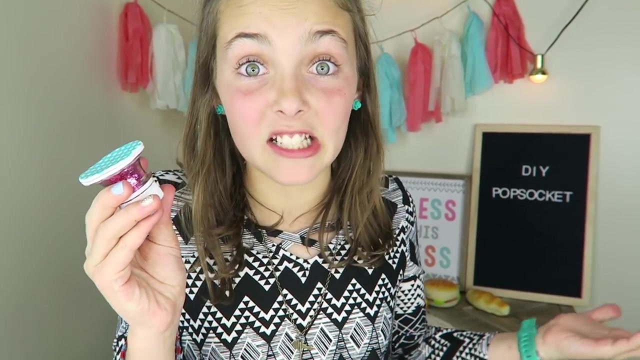 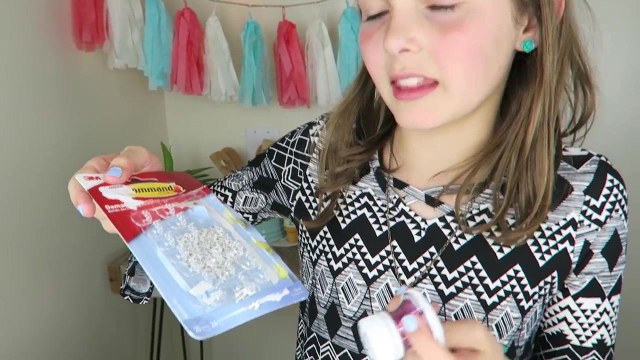 There we go. It's so cute and it's so smooth. All that's left to do is attach it. So if you want this to be like kind of a temporary thing, you can use these stickies that I use for my locker. 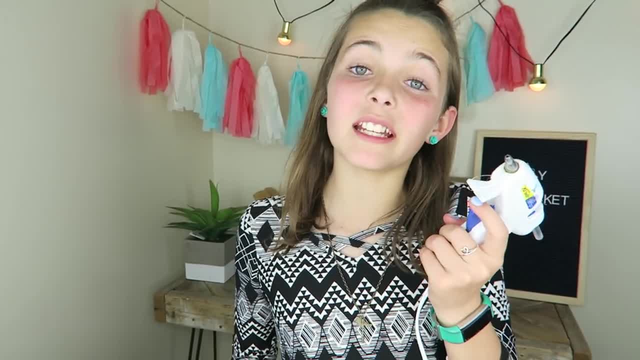 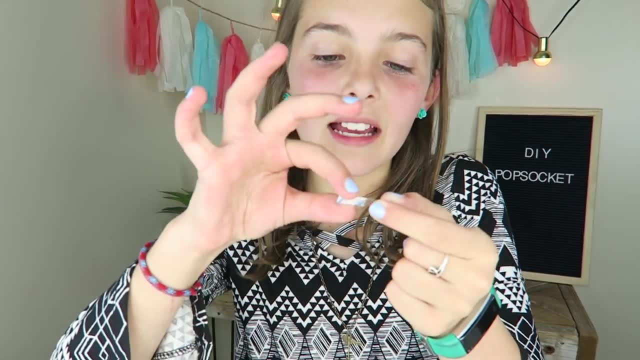 Go watch that video next. But if you want it permanent, you can just hot glue it. I'm just going to use these hooks, So these stickies that come with it. One side is for the wall And one side is for the wall. 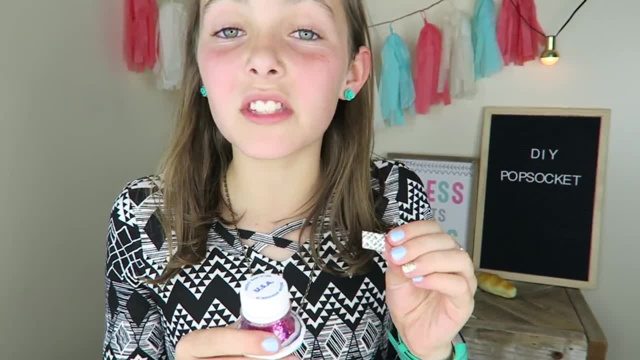 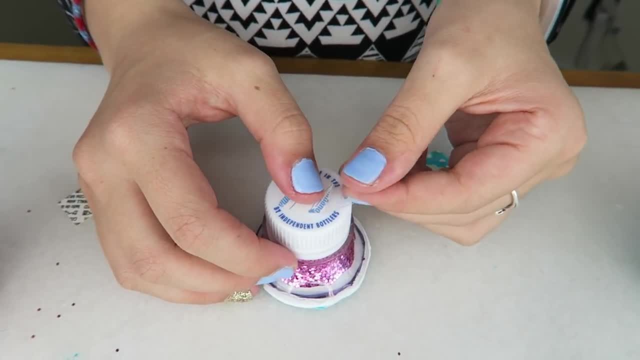 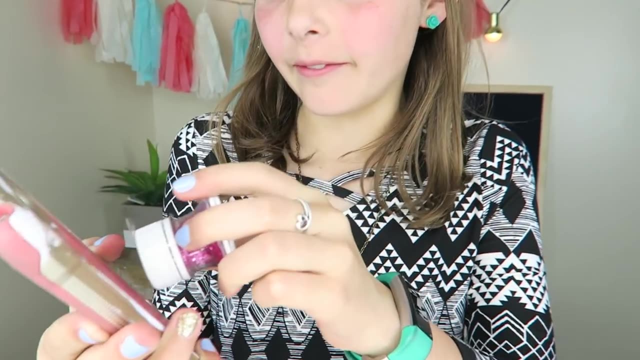 And one side is for, like the hook, But we're going to use it for one side for the phone and one side for the pop socket. Now I'm just going to put the phone right on. Now I'm just going to press it. 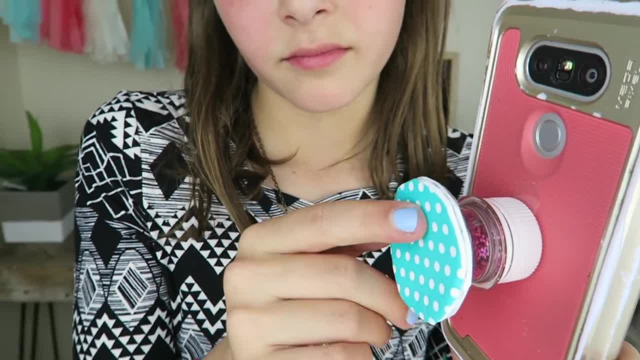 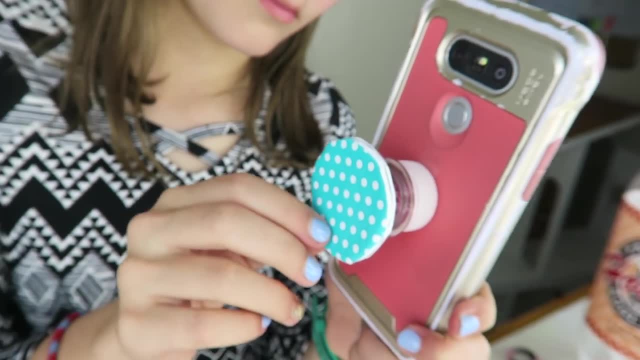 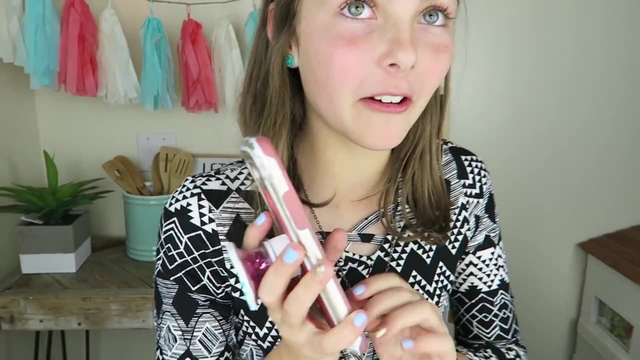 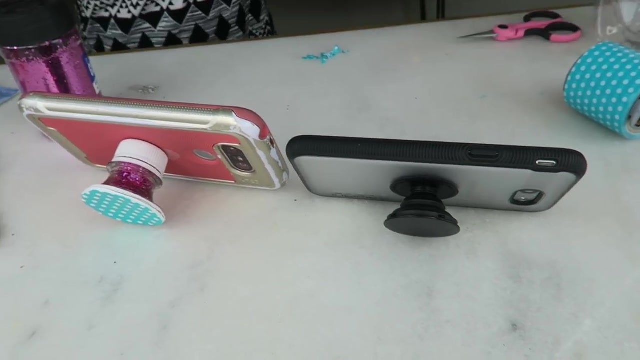 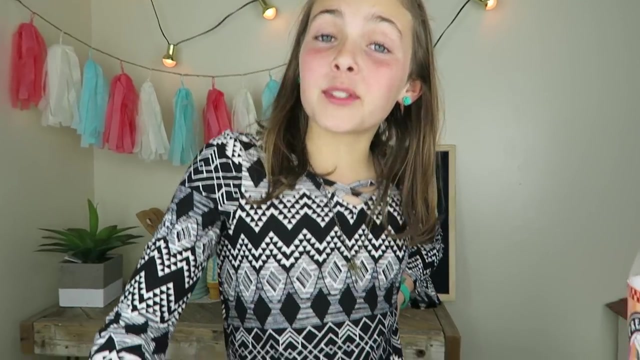 Check it out. I can take a selfie without dropping my phone And I can set it on the counter to watch a movie. My pop socket can't squish down like my brother's, But I'll be trying to fix that in another video. 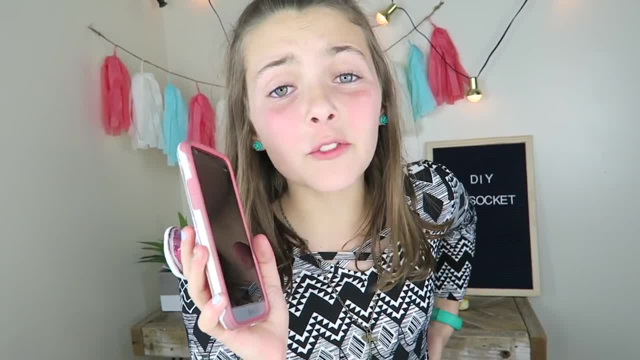 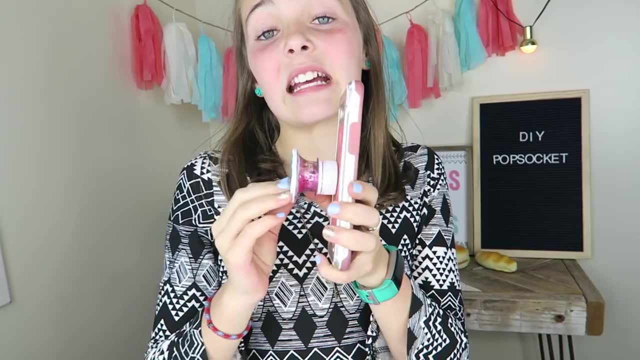 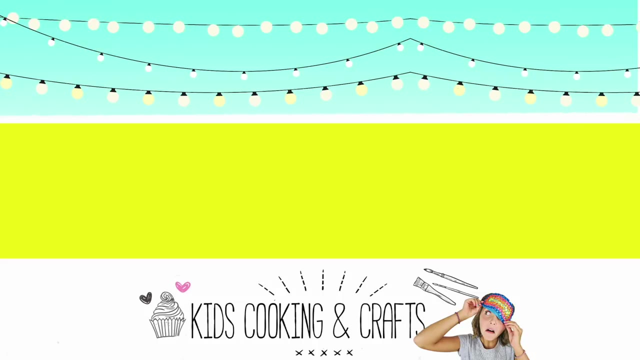 So stay tuned. Thank you, guys. so much for watching. Don't forget to like, subscribe and comment down below what color of glitter you would use. See you guys next time. Bye, Bye, Bye.